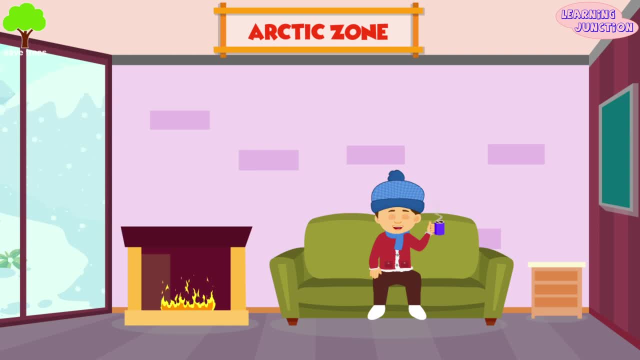 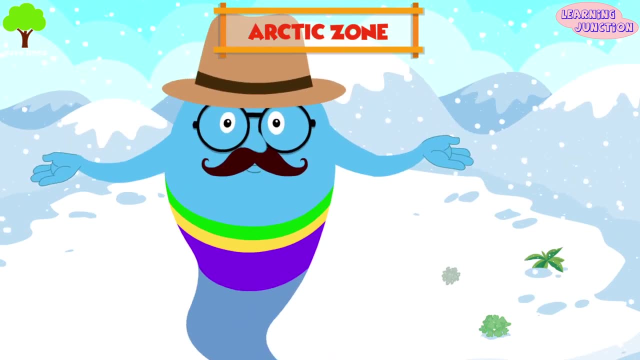 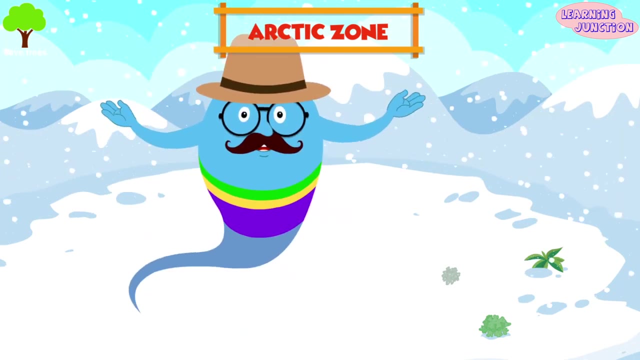 In the Arctic, the average winter temperature is around minus 22 degrees Fahrenheit. At the South Pole, it's even much colder. It's even too cold for trees to grow. You won't find trees in Antarctica, But some types of small shrubs, lichens and algae somehow grows in this climate. 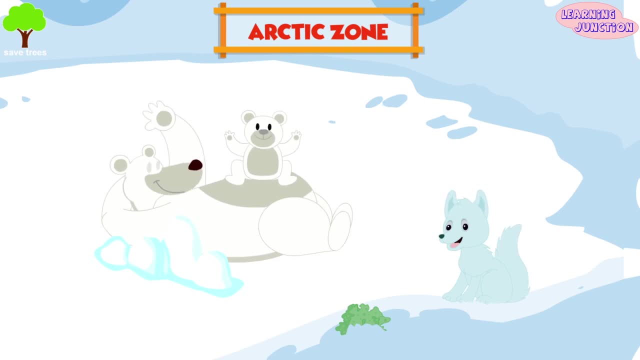 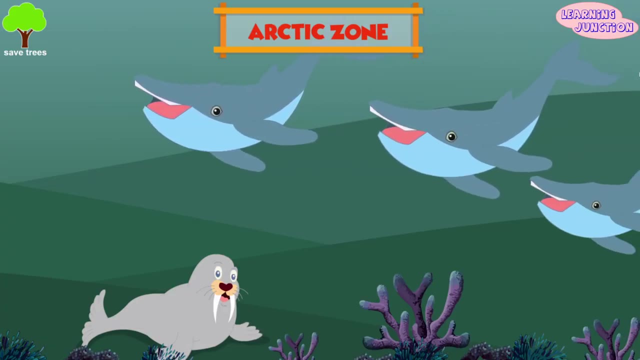 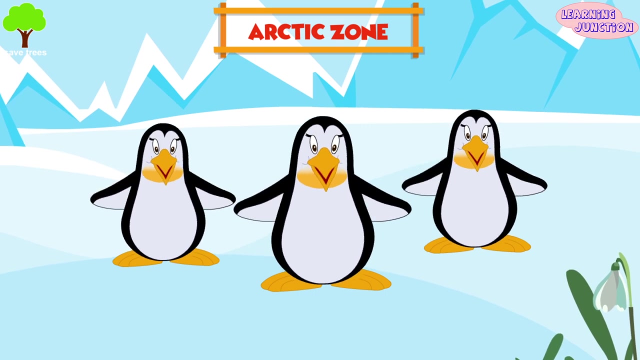 Animals like polar bears and arctic foxes are adapted to the extreme weather of the Arctic zones. Humpback whales and walruses live in the Arctic Ocean. Different types of penguins, including the emperor penguin, live in Antarctica. Now let's visit the tropical zones. 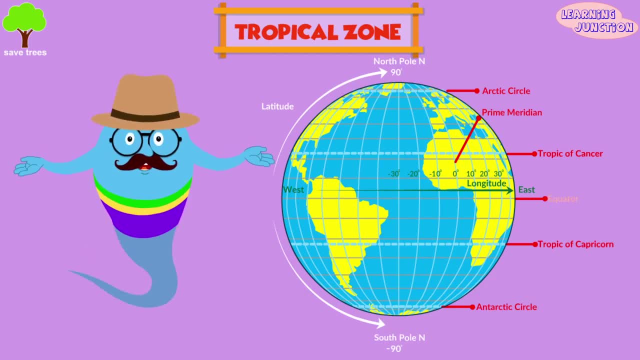 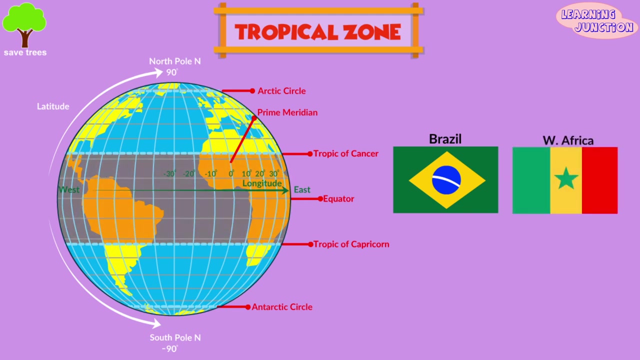 These zones are the region of the Earth near to the equator and between the Tropic of Capricorn in the Southern Hemisphere and the Tropic of Cancer in the Northern Hemisphere. The tropical zone includes the Amazon Basin of Brazil, West Africa's Congo Basin and the rainforests of Indonesia and Malaysia. 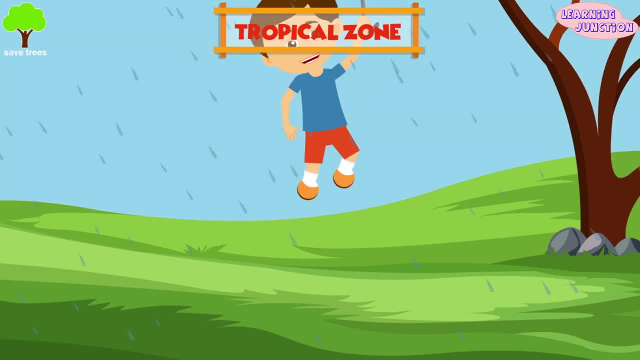 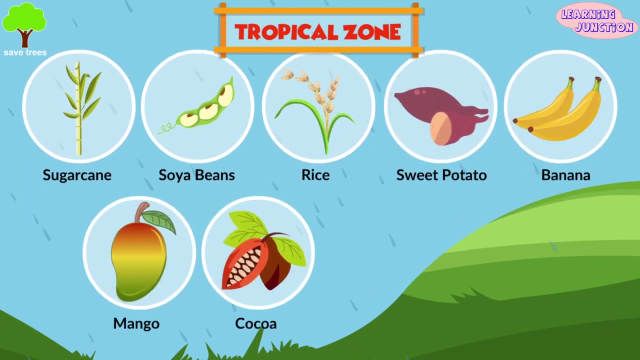 This climate zone experiences high temperatures all year round and lots and lots of rain, And so the climate of the zone is very humid: Sugarcane soybeans, rice, sweet potatoes, bananas, mangoes, cocoa, tea and coffee, etc. 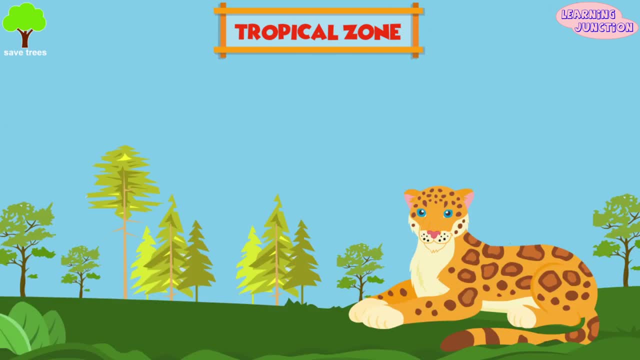 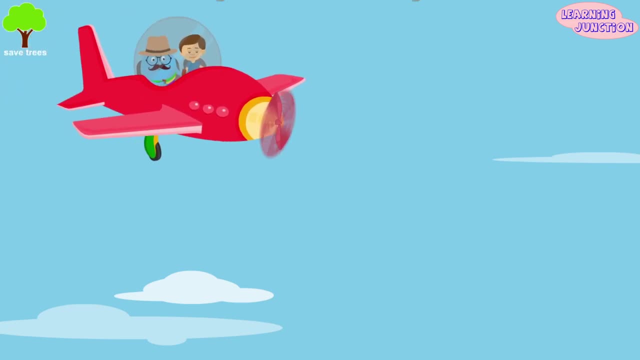 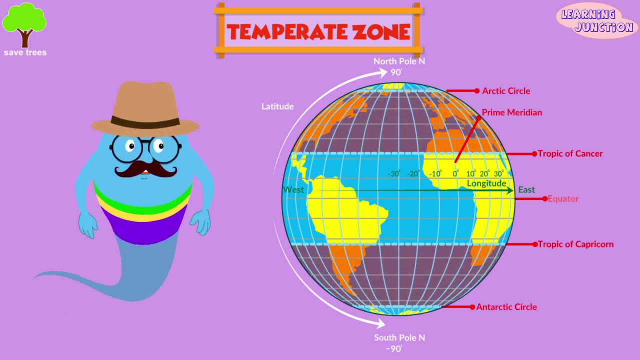 are grown in this zone. The climate of the tropical zone is perfect for animals like jaguars, anaconda, etc. And now it's time to visit the temperate zones. These zones are usually midway between the equator and the poles. This region includes most of Western Europe. 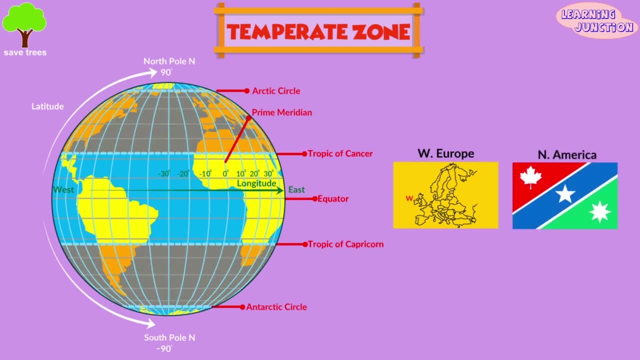 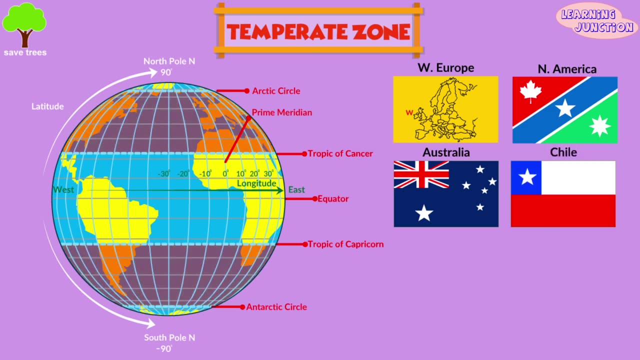 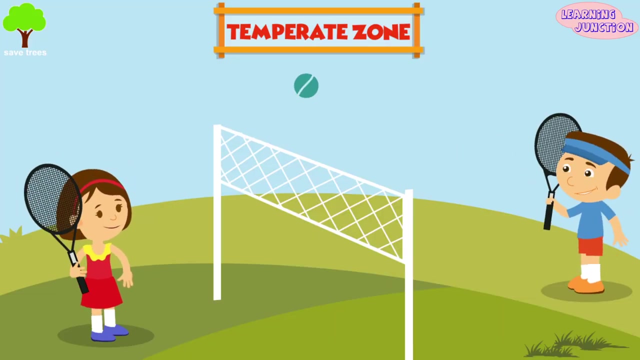 and some areas of the North America's West Coast. in the Northern Hemisphere, In the southern half of the world, the southeast of Australia, some areas of Chile and Argentina and New Zealand have a temperate climate. The weather isn't extreme in this zone. 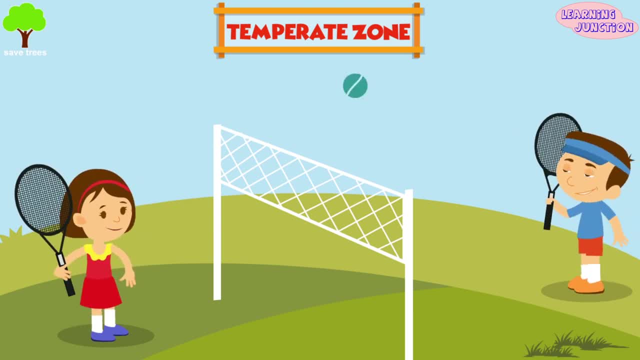 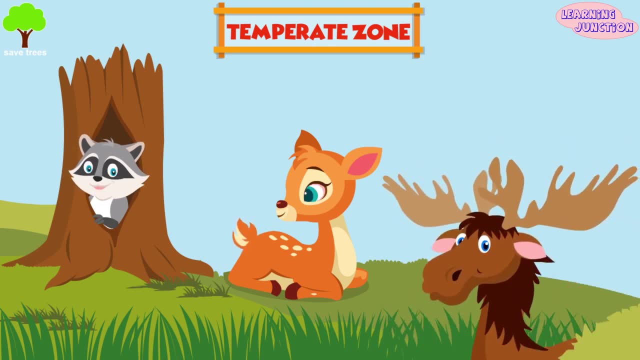 They usually have warm, dry summers and short rainy winters. A wide variety of animals like raccoons, deer and moose live in temperate forests. In temperate regions you can easily see trees like pine, deodorant fur and spruce.